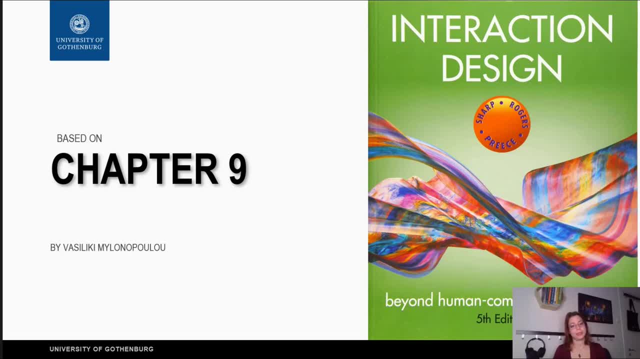 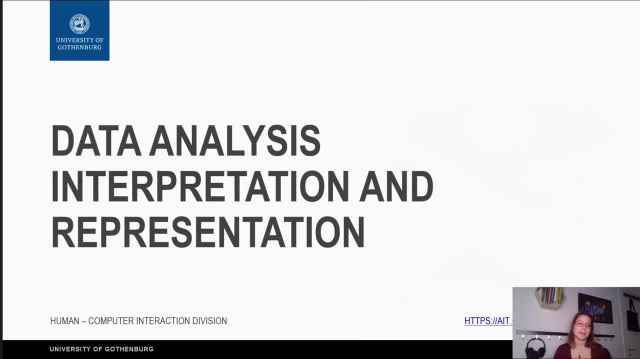 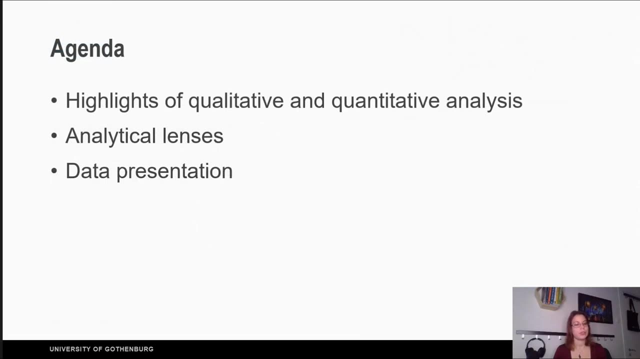 Hello and welcome to the video related to chapter 9 of the book Interaction Design Beyond Human-Computer Interaction, the fifth edition. This chapter has the name Data Analysis, Interpretation and Representation. In this video we will talk a bit about the highlights of quantitative and qualitative analysis. 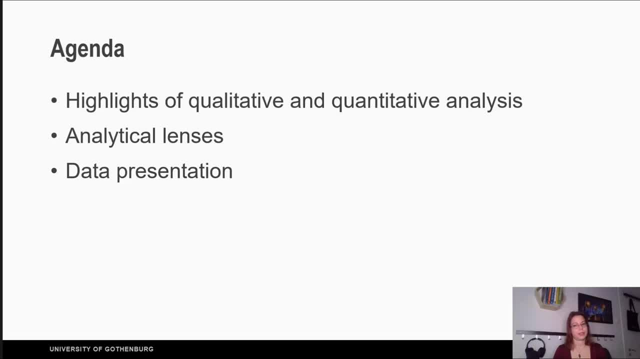 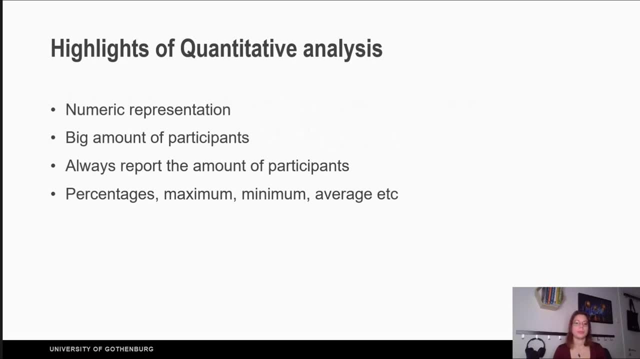 analytical lenses and data presentation. Highlights of quantitative analysis. Most possibly, you will have numerical data or your question will be related to numerical data. For example, how many times the word empathy exists in this text? The participants that you may have. it may be hundreds, and you should always. 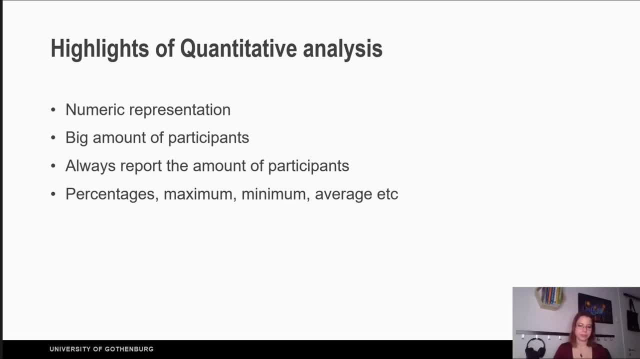 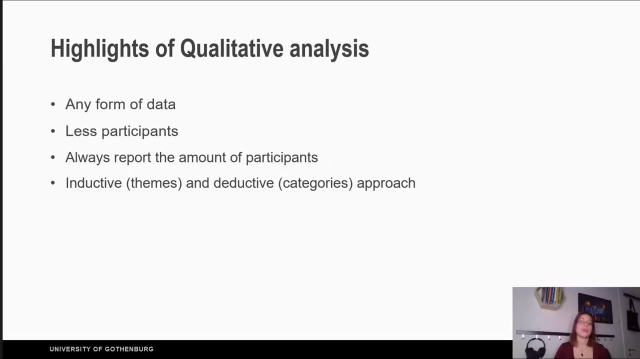 report them. The amount of participants that you have and what you will look for most possibly will be some kind of percentage, minimum, maximum, average, mean, and you should have a basic knowledge of statistics For qualitative analysis. the data have different forms, so they can be textual, they can be audio, they can be. 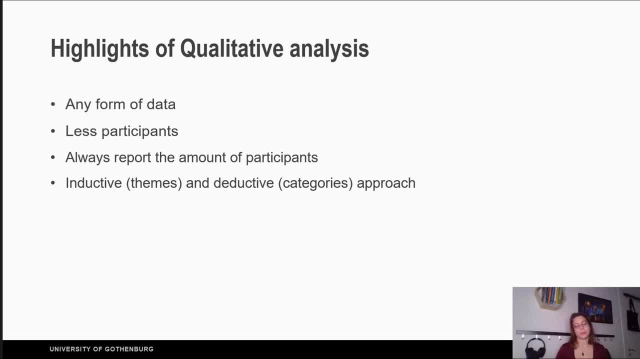 visual. The data are richer and, for practical reasons, to analyze the this rich data, you have less participants than in quantitative research. however, you still need to report how many participants are in your research and to analyze the data, you can use two approaches. the first approach is to look at the data and, based on what the data tell you to 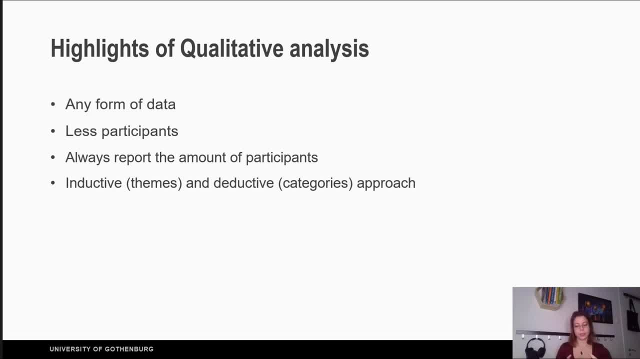 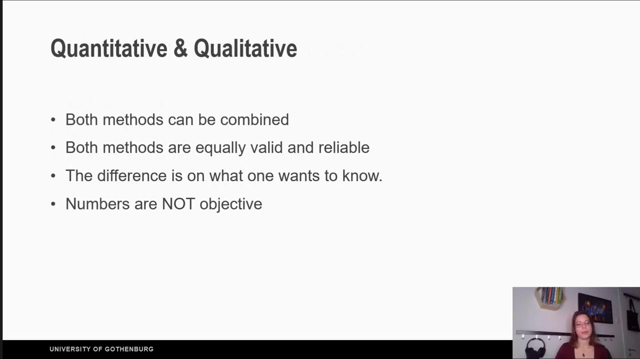 create clusters and small themes based on data that they relate to each other. the second approach is to have predetermined categories before you collect the data and when you have the data, you can categorize them into these categories: quantitative and qualitative. both methods can be combined, both methods can be used. both methods are equally valid and reliable. 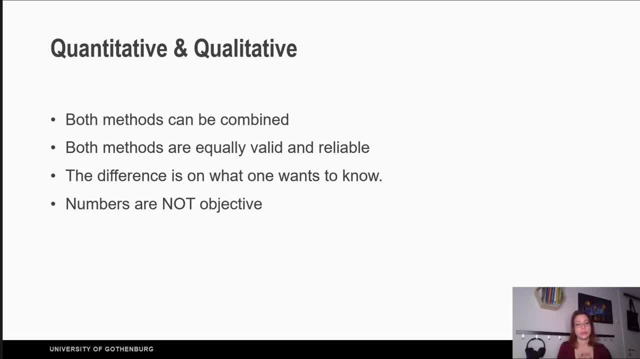 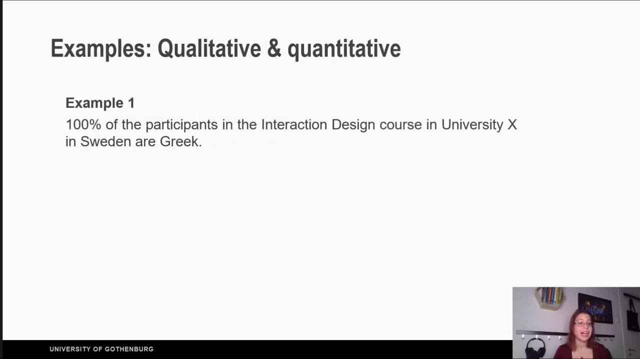 it is only the matter of what you are looking for and what is your question. what do you want to know? You shouldn't think that numbers are more objective than the language. I will give you some examples. Example 1. 100% of the participants in 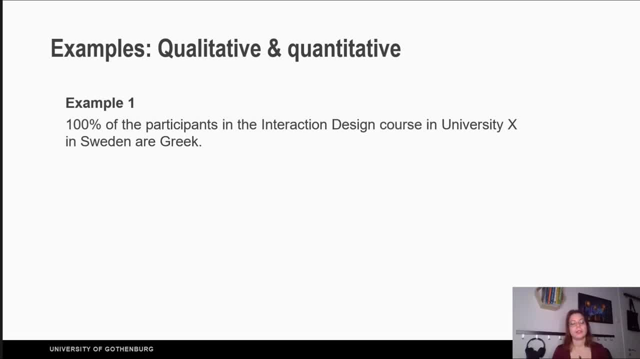 this course are Greek. As you can see, it's a big amount of students that are Greek, even though the course is given in Sweden. If we knew all the data here, you would see that this hundred percent is only to two students. You can definitely manipulate the numerical data if you want to. Another example that 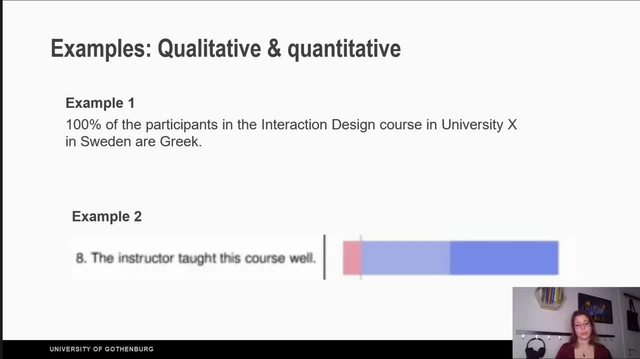 quantitative data are not sufficient is when you give feedback. For example. here we see a question. The instructor thought this course well, There were some people who said it was not good. So you can see you aren'tnt perfect Your forwards. think that yourself as well, and that these parents r find your way around. the examples. Please, you should ask questions. if you know the numbers, You, you can communicate a slightly different. I take a little more if you do a lot. Now, for example, if you want to be an expert, I can show you these words that are: 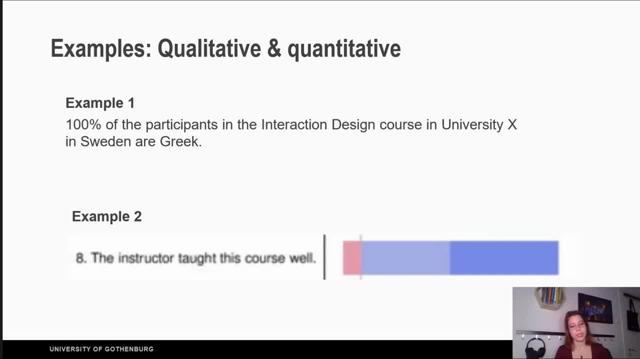 that said no with the red, some people that they said okay, some people that they said very well, This as an instructor doesn't give me any value. I would need to know what I did wrong in order to fix it. So in that case, probably it would have been. 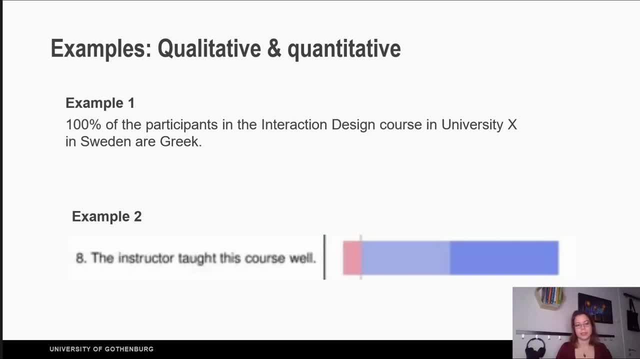 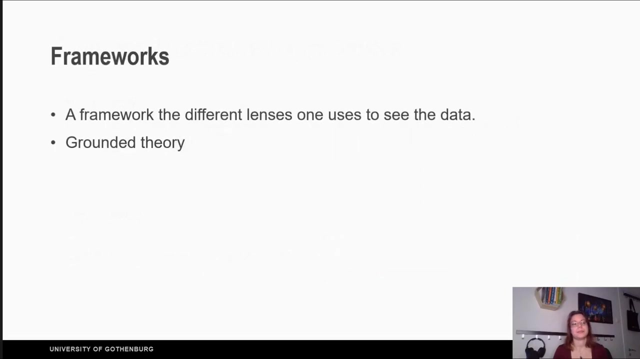 better to use qualitative research. Similarly, in the first example, if the students are only two and we need to include them in some research, we need to justify why we will choose quantitative instead of qualitative, since the sample is too small. Analytical lenses- The analytical lenses are frameworks. There are different. 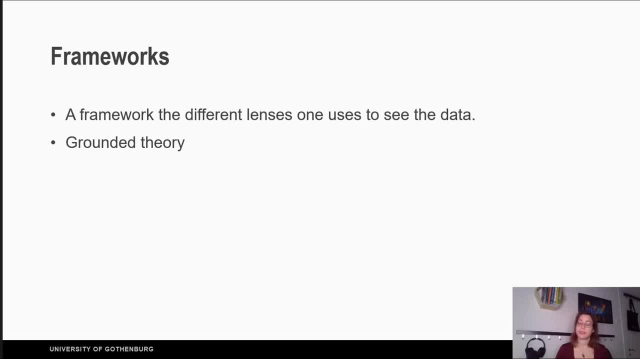 frameworks out there, For example, the discourse analysis framework, You see, through your data, the power relationships between the people, between your participants. So you can see the power of relationships between the people, between your participants. So you can see the power of relationships between the people, between your participants. 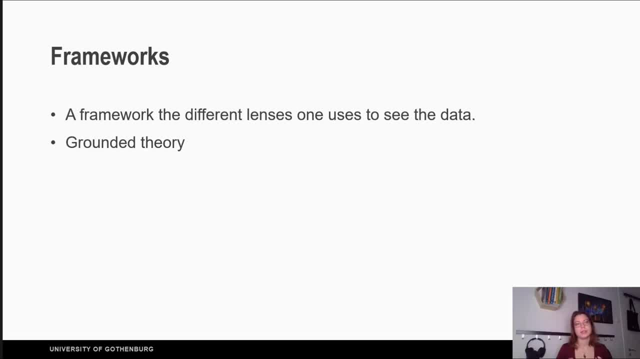 While when you use content analysis, it is to figure out how frequent, for example, a word is referenced in a text. If you want to create a new theory, most possibly you will use the grounded theory In academia. it is important to specify which definition of grounded theory one uses, as it can be a reason of